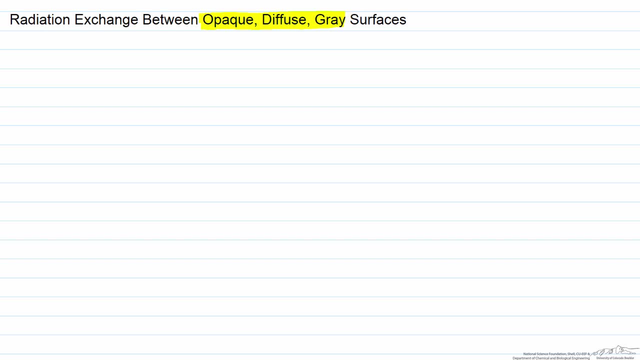 So how do we do that? Well, the total rate at which radiation reaches the surface from all other surfaces is going to equal. the summation from J equals 1 to N, where N is the number of surfaces, the view factor from that one surface to the original surface. 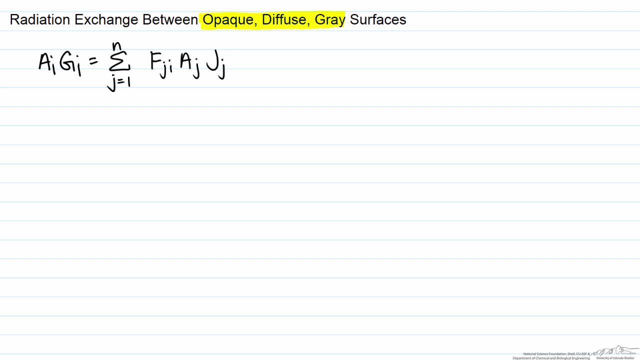 times the area of that surface, times the radiosity. By the reciprocity rule which was discussed in the screencast on view, factors F sub J: i times the area sub J is equal to F sub i, J times A sub i, And this will allow us: 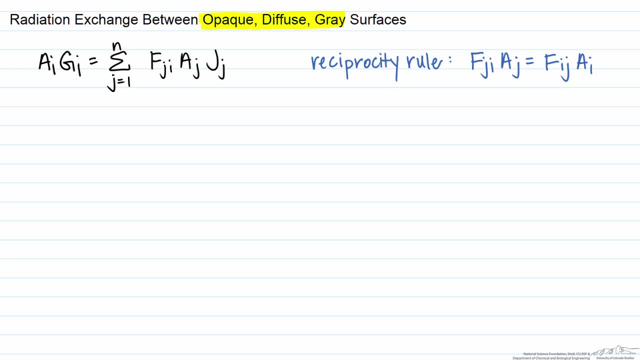 to cancel our A sub i from both sides of the equation. So now we're left with our irradiation equals the sum for J. equals 1 to N F sub i, J times the radiosity from surface J. Now let's go back to our equation. 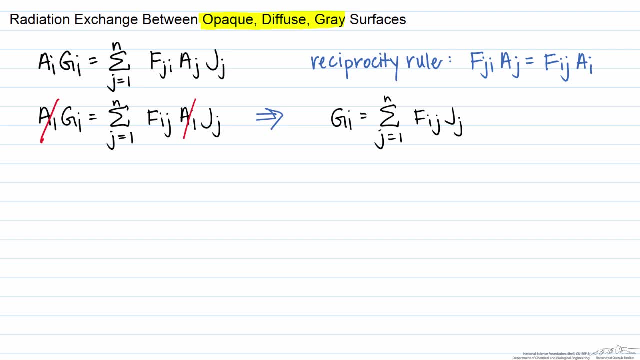 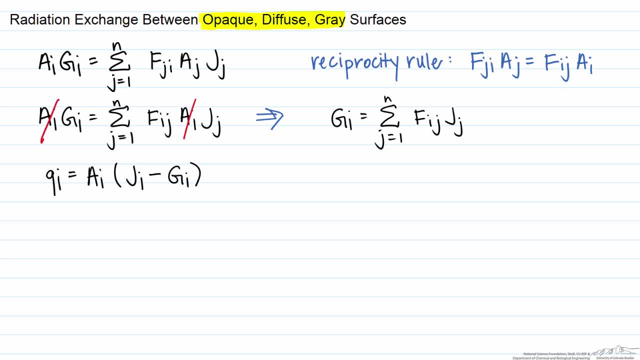 radiosity. The emission value if the irrideant radiation is lengthwise from one surface to another will look like. represents what the x x선 wave is. Subtitles by the Amaraorg community. write it in terms of this heat transfer, and this is equal to our area. the radiosity from: 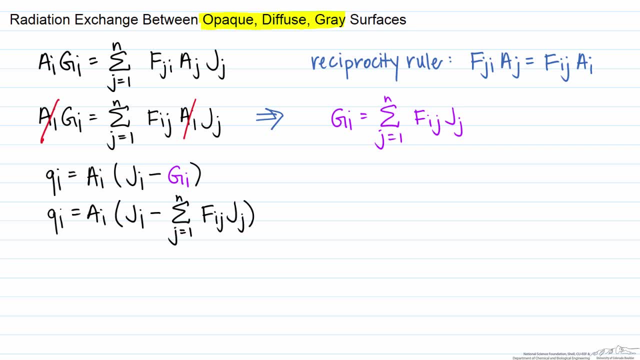 i minus the summation from j equals 1 to n. f sub ij times j sub j. Now we're going to use a little mathematical trick. The sum of the view factors in any enclosure has to equal 1.. So now we can put that in front of our j sub i, and so this can be finally: 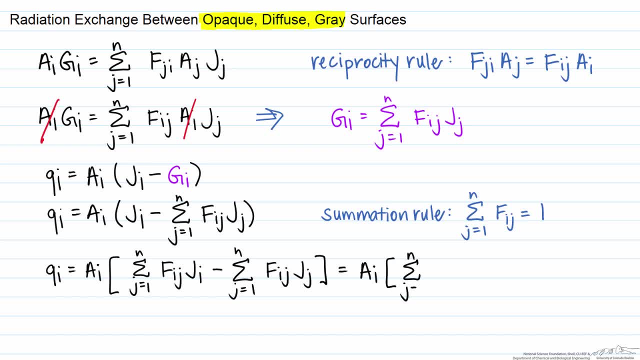 simplified our area times, the summation from j equals 1 to n, The view factor between them and the difference in radiosities. This can also be considered. the summation for J equals 1 to N of Q, from I to any one of the surfaces J. So this would: 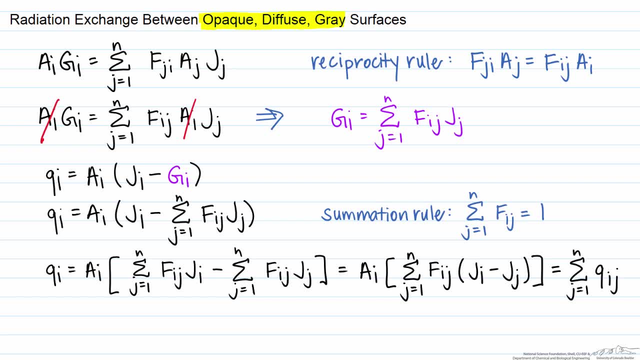 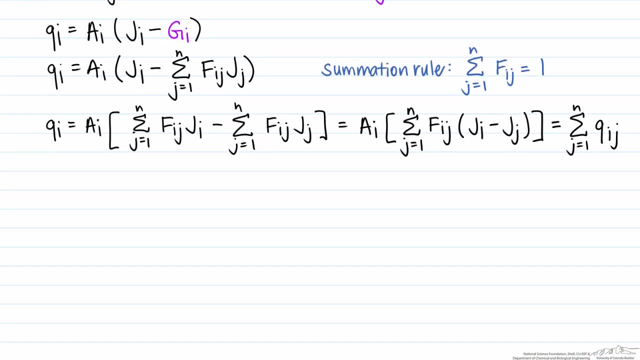 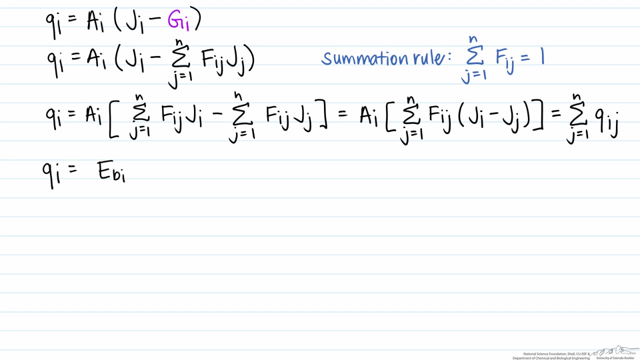 be the net rate of radiation transfer from I to the sum of the radiative exchange with other surfaces. Now we can also write Q I as EI minus Jr, where E is the emissive power of black body, One minus I emissivity divided by the emissivity times the area of the surface, and therefore this: 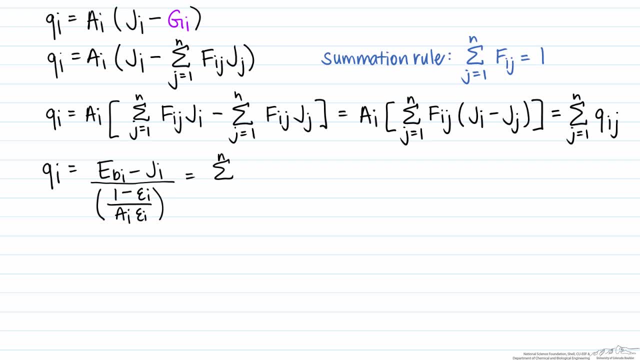 is going to equal: the sum from j equals 1 to n, the difference between the radiosities of each surface- a sub i, f sub i, j- to the minus 1.. So I just rewrote this equation And again, this can be used for exchange with any number of the opaque, diffuse gray surfaces. 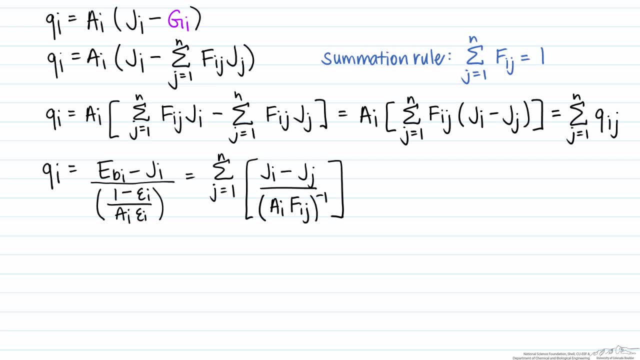 in an enclosure And it might be easier to visualize it like this. So here's a graph of our radiative heat transfer rate and it goes into a network And we start with this emissive power of a black body and again, this is part of the driving force where the